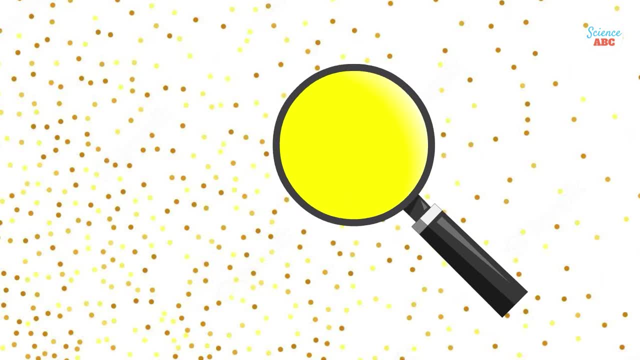 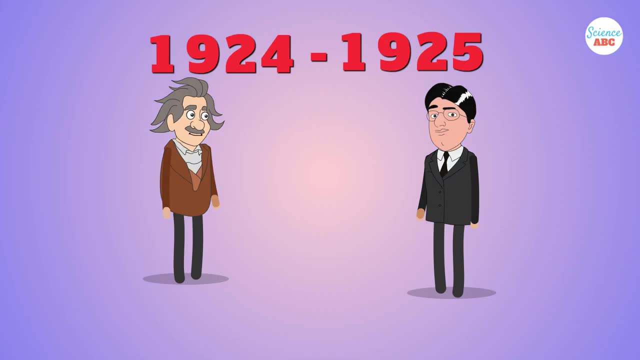 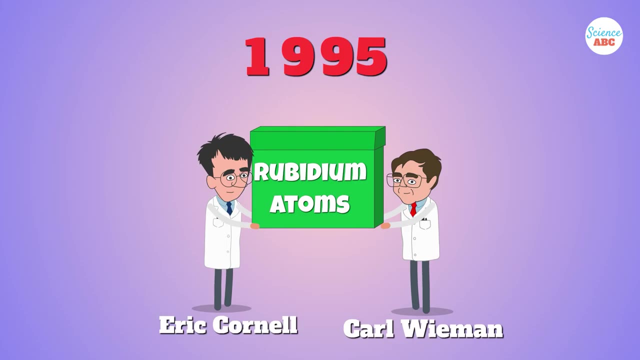 If you were to measure their location at this point, you would observe a blurred ball rather than individual atoms. The Bose-Einstein condensate was initially predicted in 1924 and 1925, but wasn't created until 1995 by American physicists Eric Cornell and Carl Viemann using 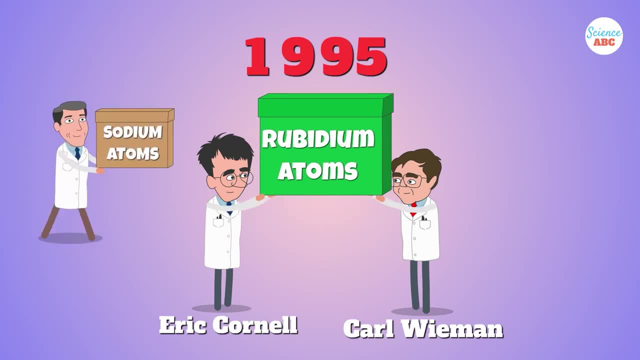 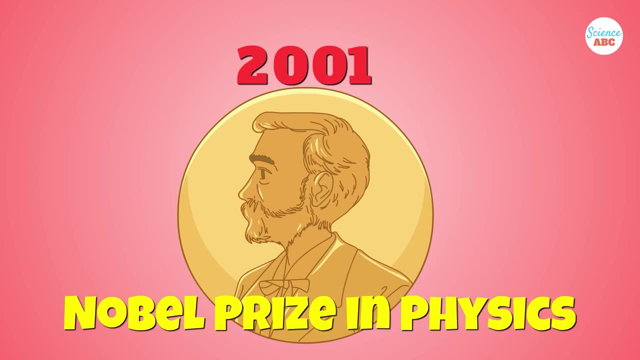 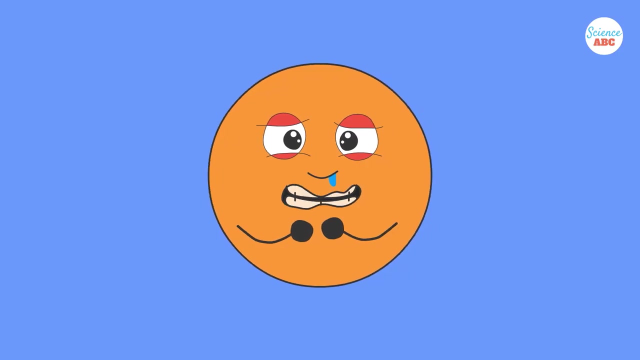 rubidium atoms. Peter Lee, a German physicist, produced the condensate the same year using sodium atoms. In 2001,. these physicists won the Nobel Prize in Physics for achieving Bose-Einstein condensation, Studying particles at near-absolute zero temperatures and creating Bose-Einstein condensates has. 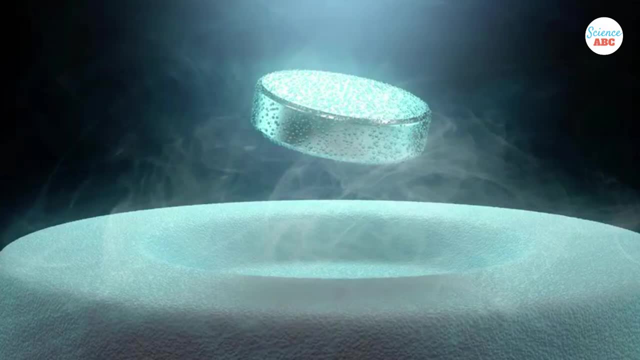 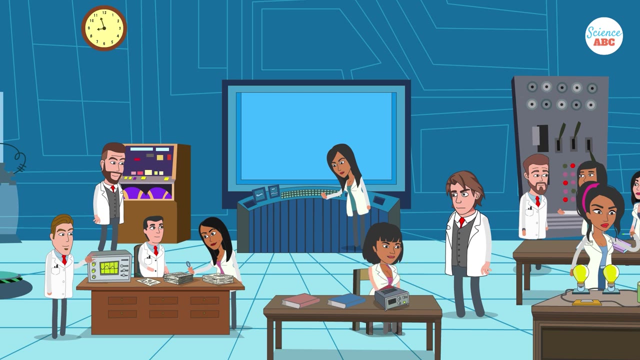 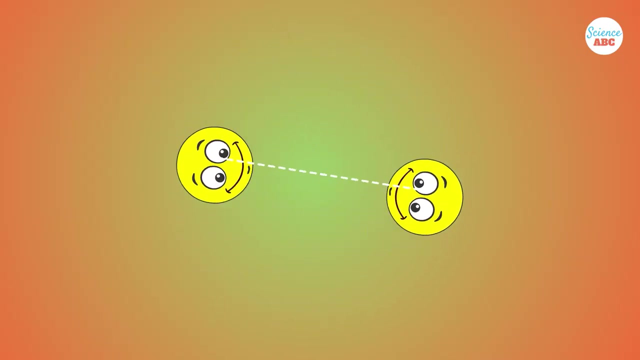 important implications in areas like quantum computing, superconductivity and scientific research. One example of how researchers use BECs is to gain a better understanding of quantum entanglement. This phenomenon in quantum mechanics explains how particles that are entangled can affect each other's state regardless of their physical distance. 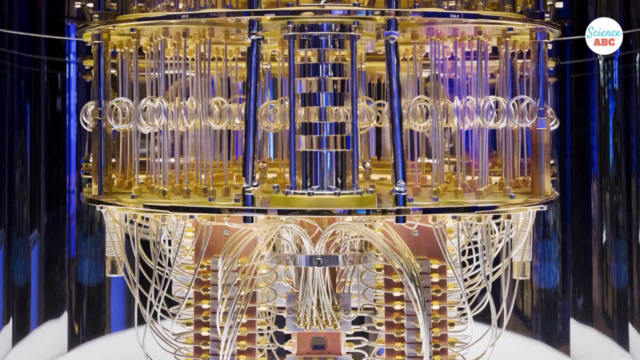 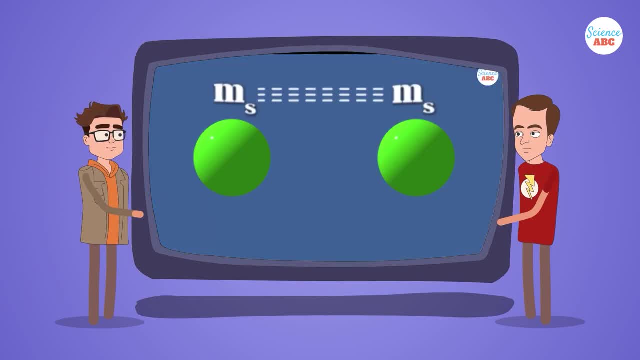 Quantum entanglement is crucial for many technologies, including the fast-emerging field of quantum computing. We have created a separate video about quantum entanglement. you can find the link in the description of this video. Bose-Einstein condensation is a phenomenon that occurs when a particle is entangled in 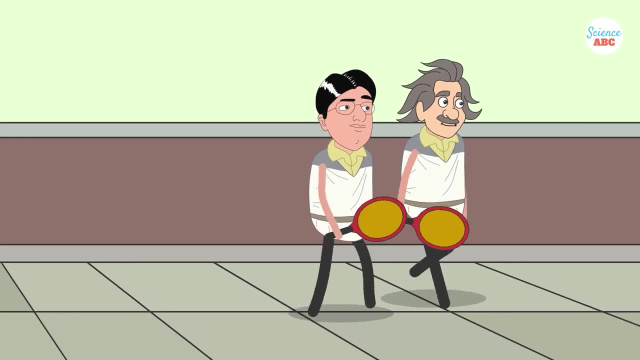 the center of a particle. This phenomenon occurs when a particle is entangled in the center of a particle. This phenomenon occurs when a particle is entangled in the center of a particle. Bose-Einstein condensates have various practical uses in precision measurement and sensing. 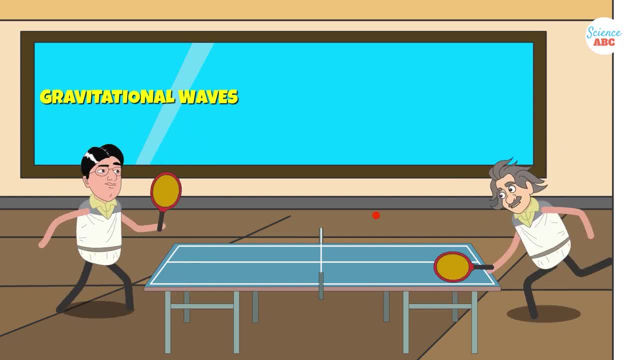 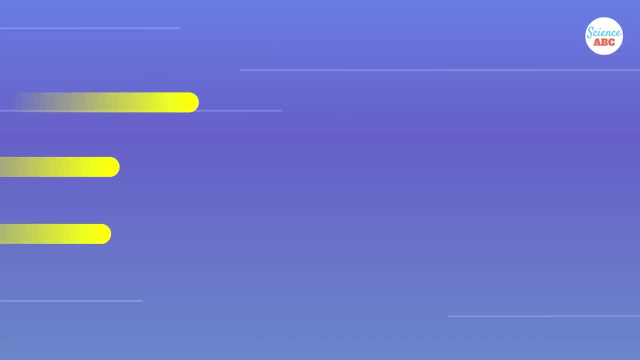 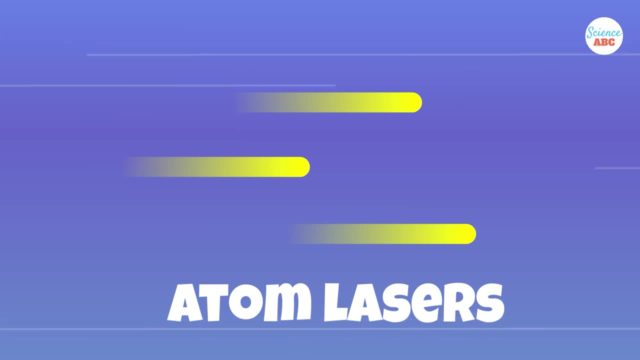 technologies which have led to advancements in detecting gravitational waves, creating navigation systems and improving magnetic resonance imaging. In addition, BECs have been used to develop atom lasers which hold great potential for the precise manipulation of atomic matter. This advancement has already aided research in quantum optics and lithography. 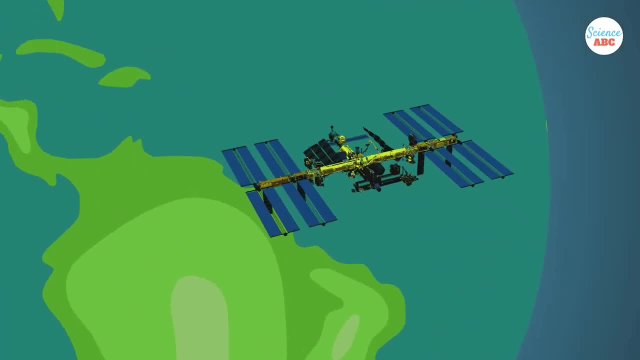 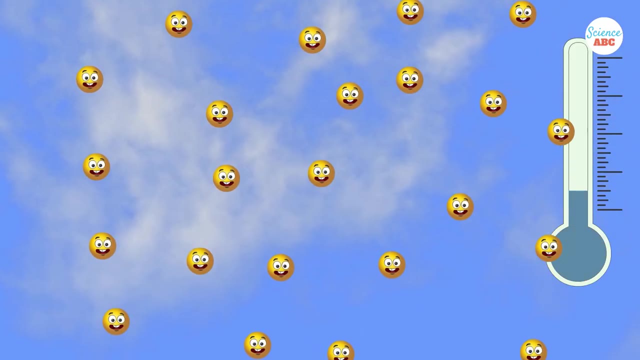 In 2012,, Bose-Einstein condensates were used to develop atomic lasers which hold great potential for the precise manipulation of atomic matter. In 2018, a groundbreaking experiment was conducted on the International Space Station: Rubidium: atoms were cooled to nearly one millionth of a degree, setting a new record for the. 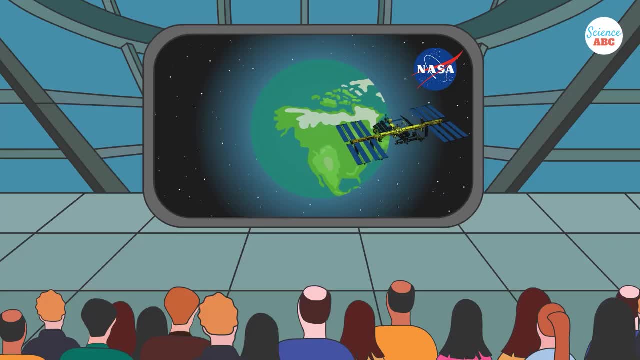 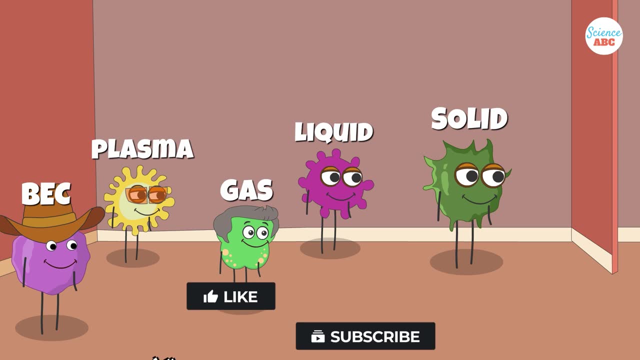 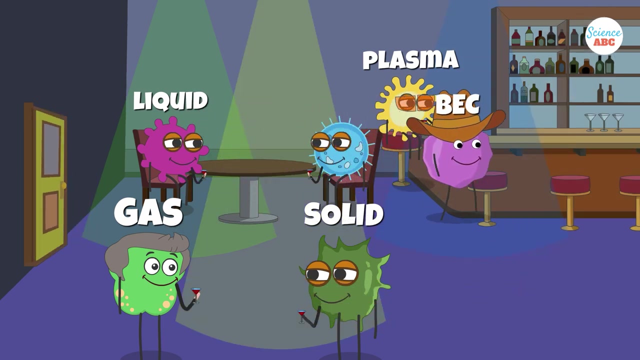 coldest experiment ever conducted in space. This experiment also marked the first production of BECs in orbit. So if the five states of matter – solid, liquid, gas, plasma and BECs – all go to a party, can you guess which one would be the coolest?